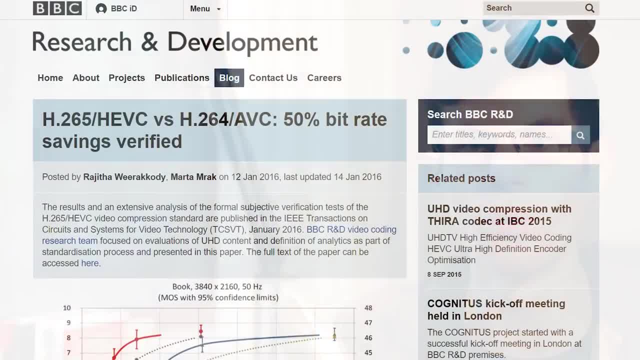 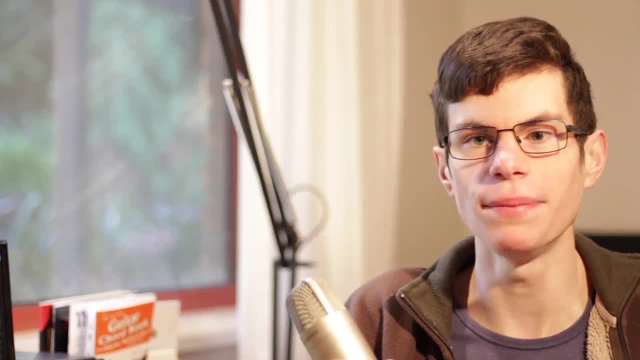 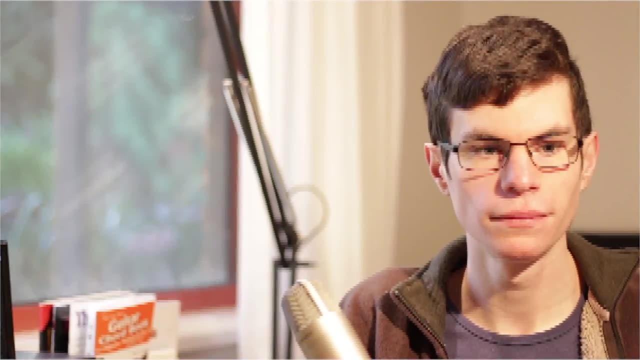 1996, to the most recent H.264.. But every new standard seems to promise the same thing: identical quality to the previous one, but at half the bitrate. So how does H.265 achieve this? Well, there's two main methods used in video compression. One is called inter-frame. 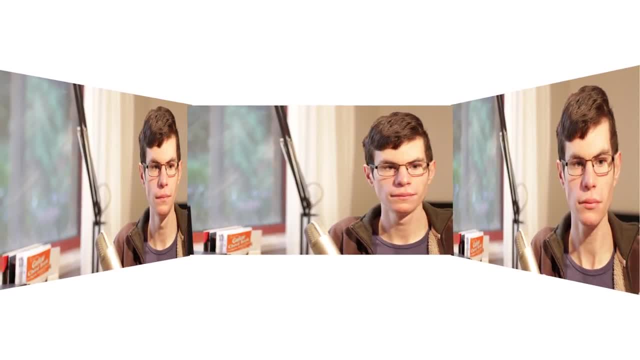 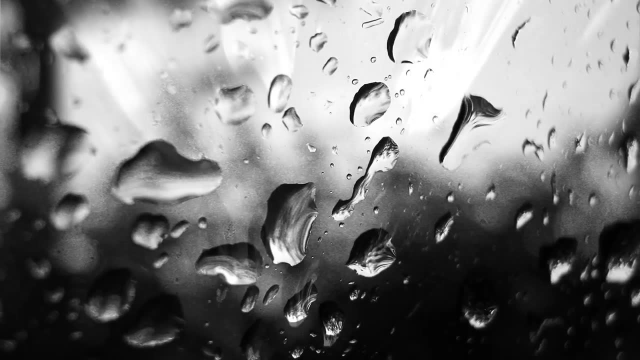 which means that the previous and future frames are compared to the current one, and we only encode what's changed. To do this, we start on an iframe, which is stored as a full image, much like a JPEG, Then we divide it into small 16x16 pixels. 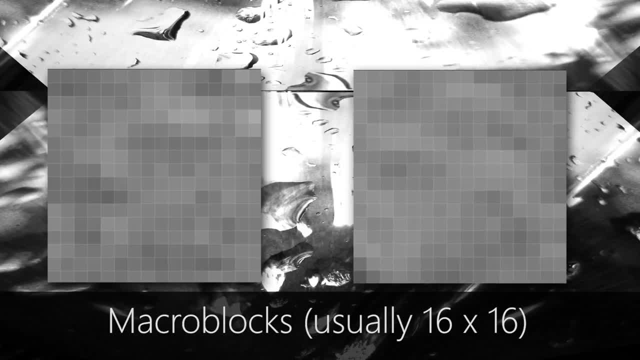 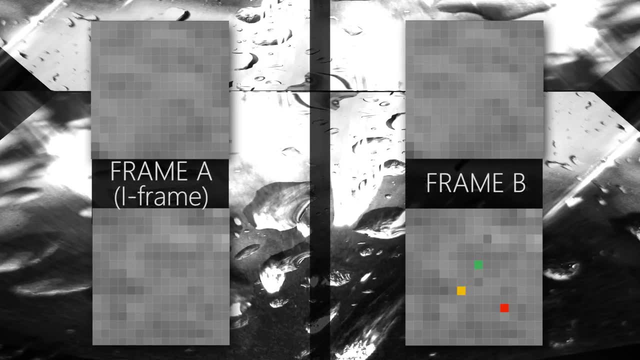 Which in the previous standard were called macro blocks. Now we're going to advance to the next frame and compare its macro blocks with that of the iframe. If there are several blocks which are roughly the same, then we give the new frame the status of a P-frame, that is, a predicted 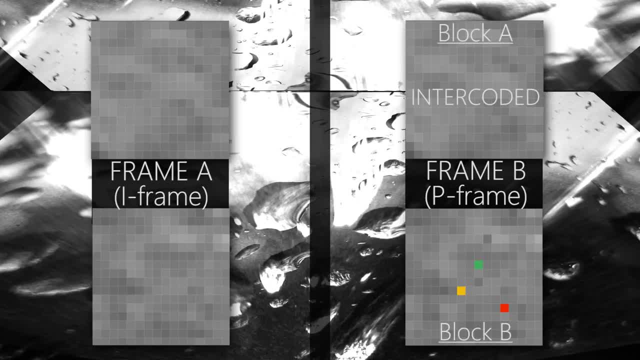 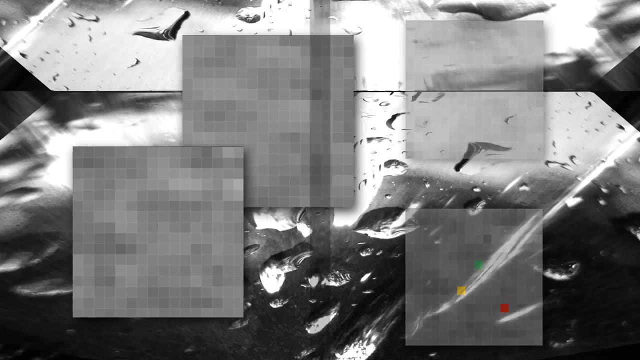 frame. This means that what we can easily do is inter-code block A, So, because it's identical, we can just bring the pixel values directly across, And then we can intra-code block B, In other words, give it entirely unique pixel values that are only for this frame. 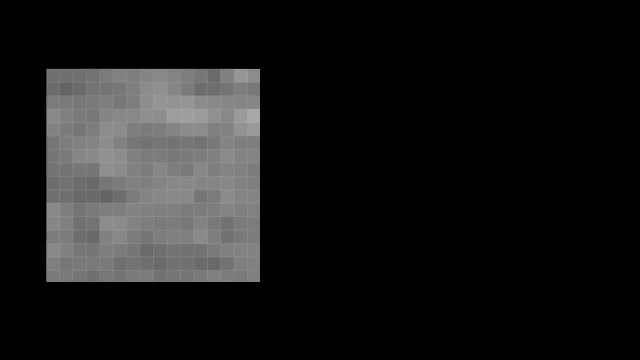 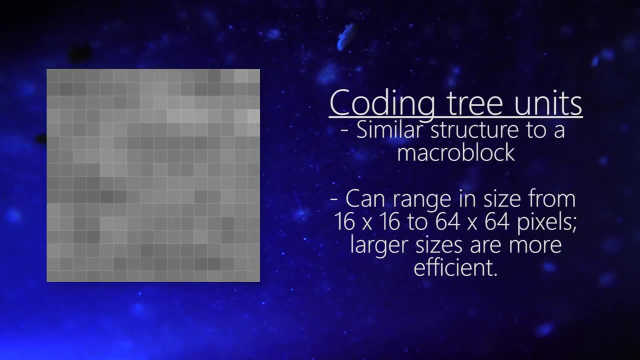 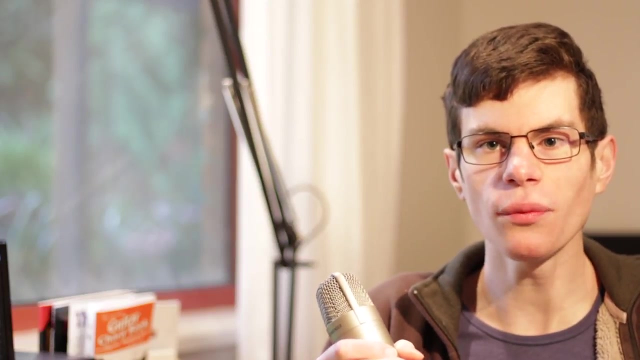 Now here is the H.265 difference. Macro blocks have now been renamed to coding tree units and they can range from the original 16x16 size way up to 64x64.. Now why is this such a big improvement? Well, you've got to remember that when H.264 was 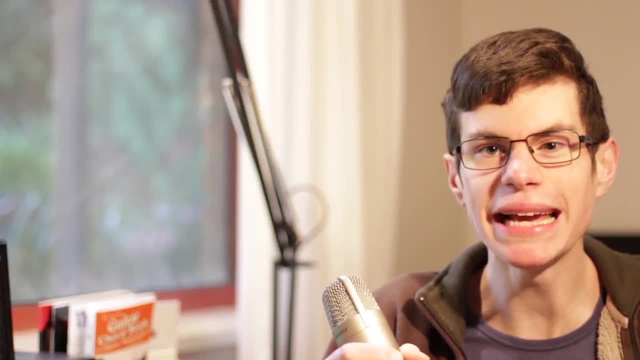 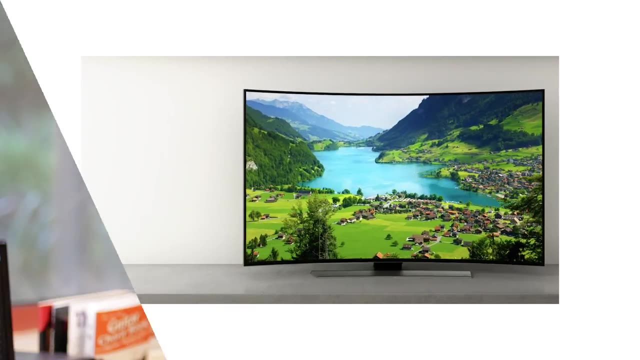 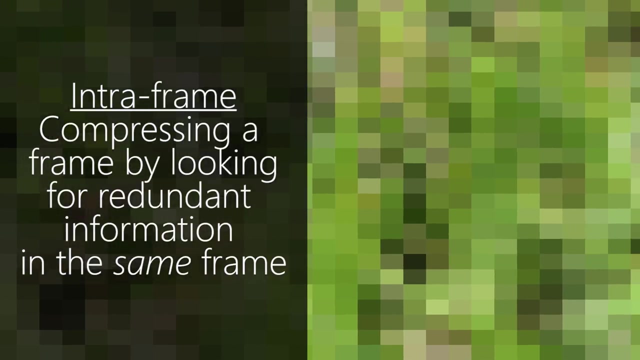 first standardised back in 2003,. video was the height of technology. Now, of course, we've got 4K and more efficient encoding is needed, And this is exactly what larger macro blocks give you Now. the second big improvement has to do with intra-frame compression, In other words, comparing areas within the same frame, and 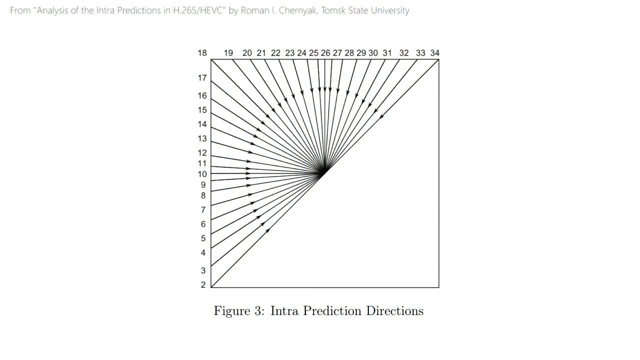 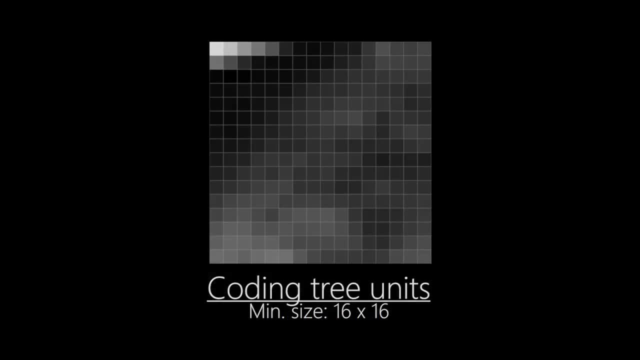 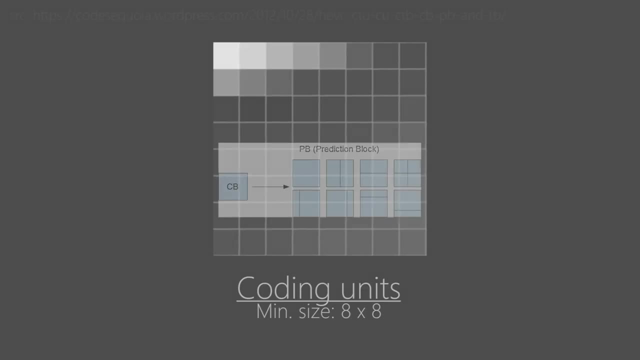 looking for redundancy And the improvement is- wait for it, the increase in prediction directions. What Well remember these things, Coding tree units, Also called macro blocks. They can actually be split further into things called coding units which can go down to 8x8 pixels, And these 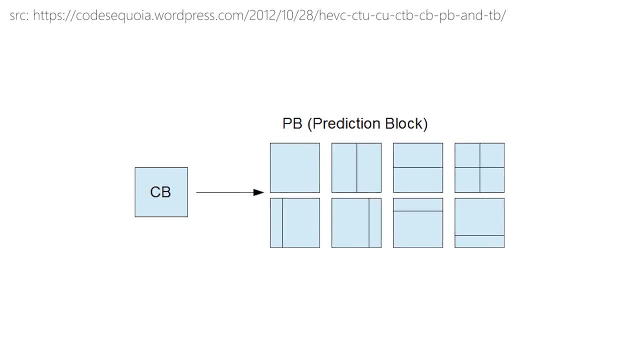 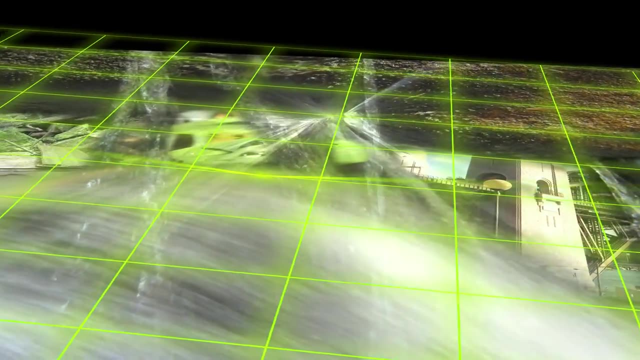 get this. they can be partitioned even further, cut up different ways, into prediction units- Why would we bother doing this? So we can mathematically generate pixel values in a block instead of storing them, And therefore we can massively reduce the size of each frame. 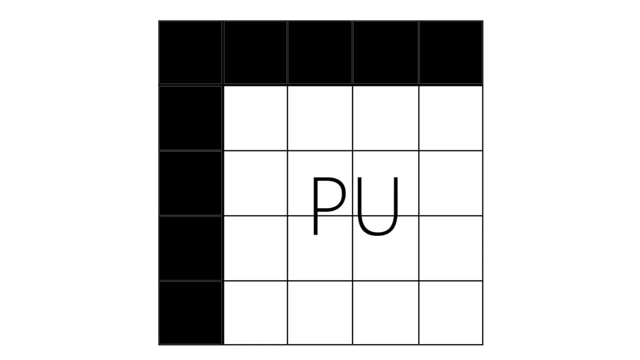 Here's how it works. I've got my tiny little prediction unit here, a little 4x4, and it's surrounded by two groups of pixels which I'll call block A and block B. Now I can actually use various intra-prediction modes on. 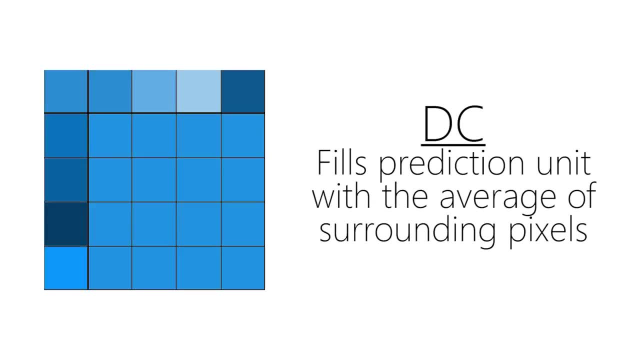 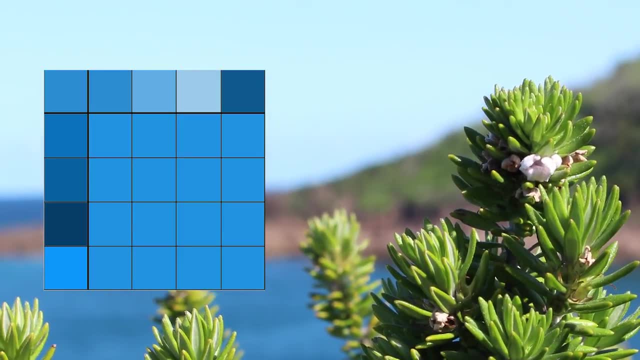 this structure. I can use, for example, DC, which will basically fill this with the average of the surrounding pixels. This would be good on an outdoor scene with a blue sky, where there's no real pattern to it. It's more of a just a single colour. Alternatively, I can use an angular. 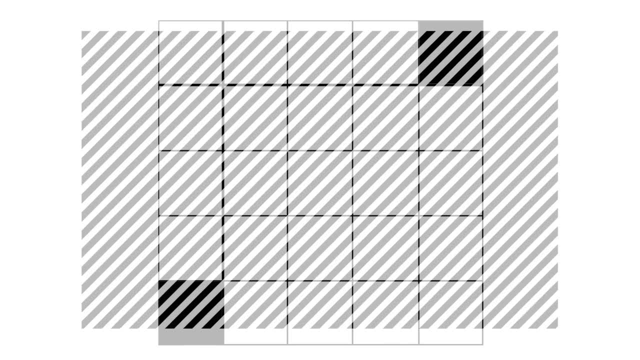 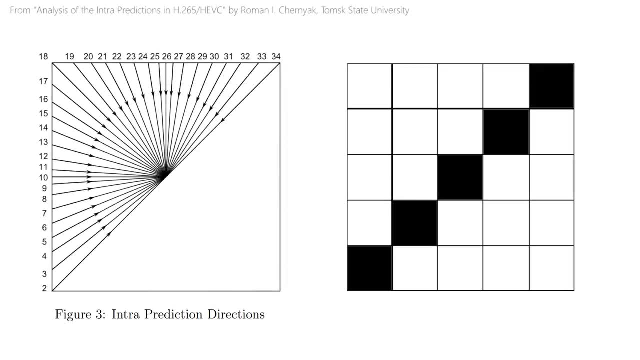 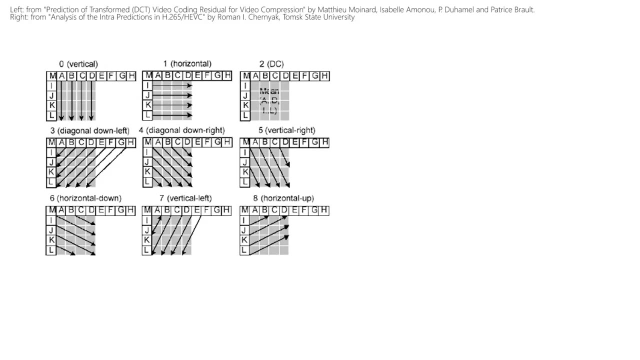 function. So say, for example, if I have a line coming down here and I want to continue it through this, I can simply point to the direction where the line is coming from and it will extrapolate or continue that trend. Now, here again, there is a difference with H.265, and it's a good one. 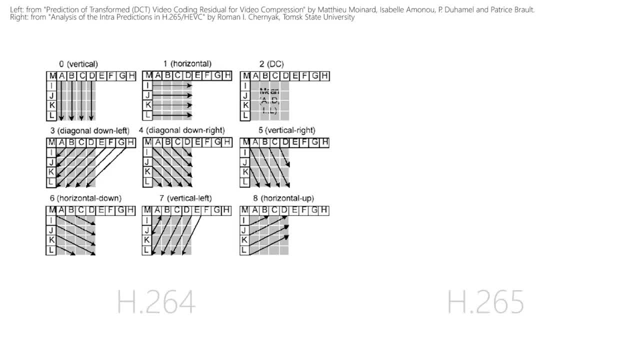 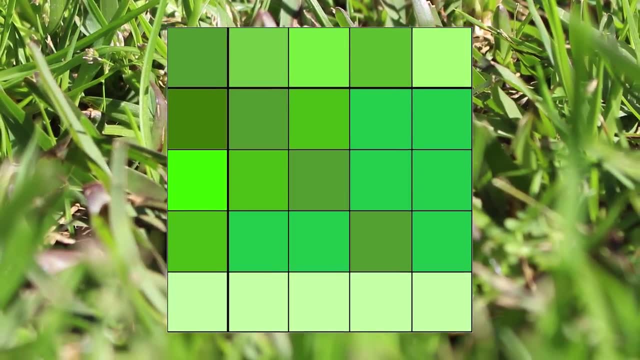 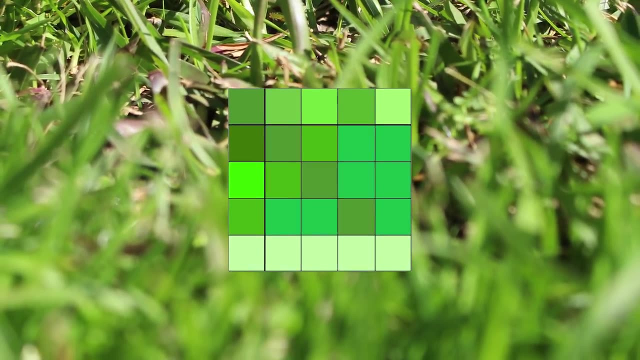 Back in the old days I only had nine prediction modes, but now I have access, to wait for it, 35 different modes. Now, the advantages to this are many, including far greater accuracy when larger block sizes are used, say, for example, in 4K video. 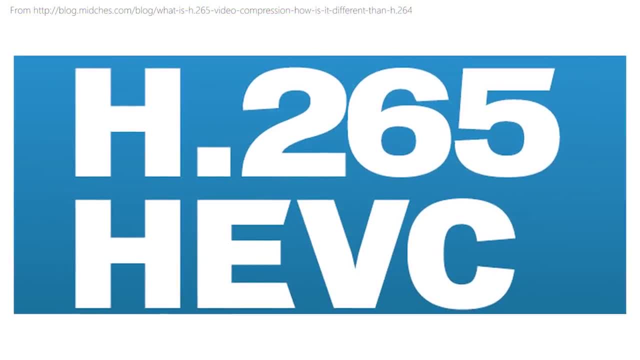 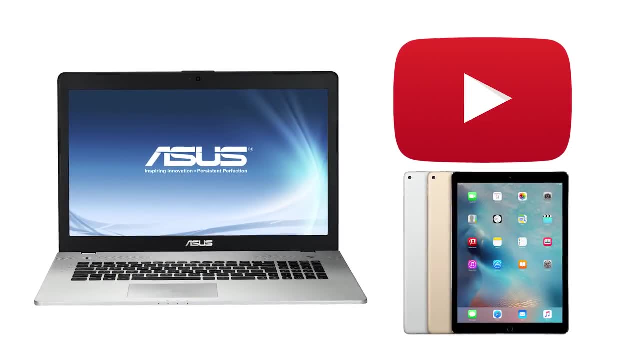 much better quality compression. So they are the main reasons why H.265 is better Bit exhausting, hey. But they're all theoretical and what you might want to know is: when can you use it? And the answer to that, unfortunately. 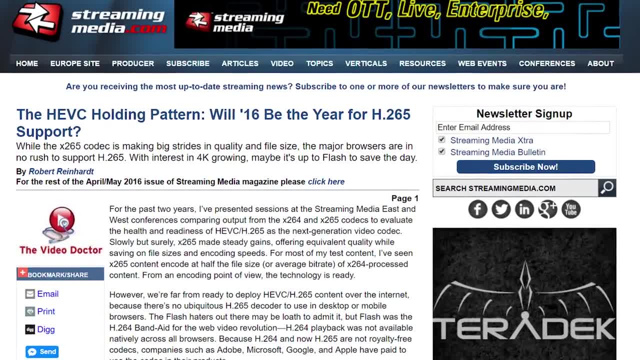 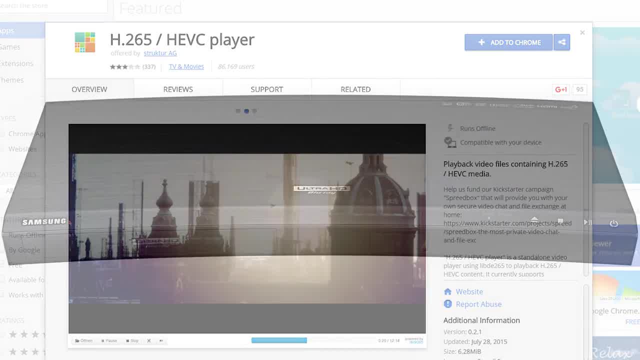 is not as often as you'd like. I mean, you can't upload videos encoded with it to YouTube and most web browsers don't support playing H.265 natively, but it's been adopted as the default codec on 4K Blu-ray and, of course, you can play it back on your PC. 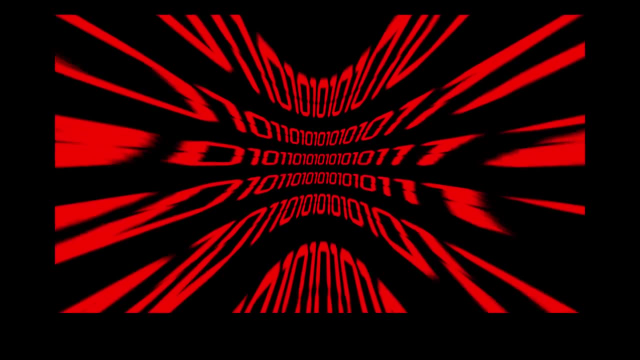 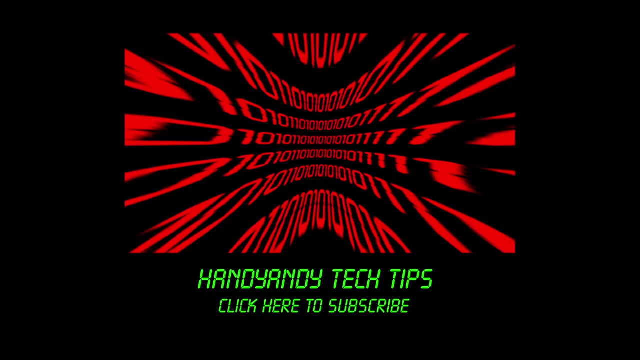 but you might need to use software decoding. Anyway, I'm HandyAndy and thank you very much for watching my video on H.265.. Please subscribe to my channel for more tech videos.